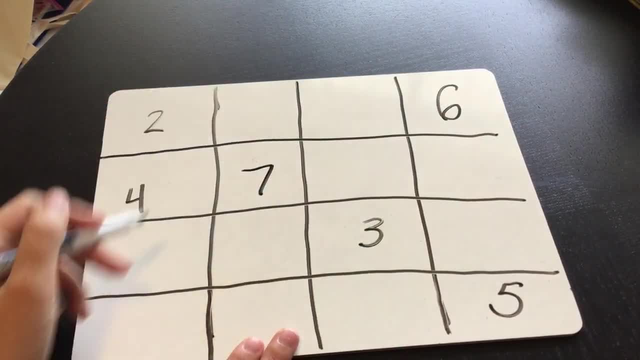 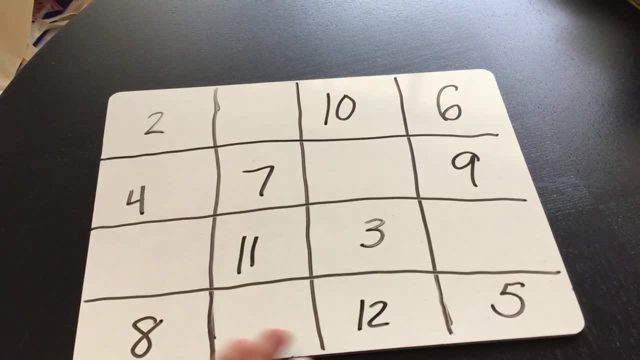 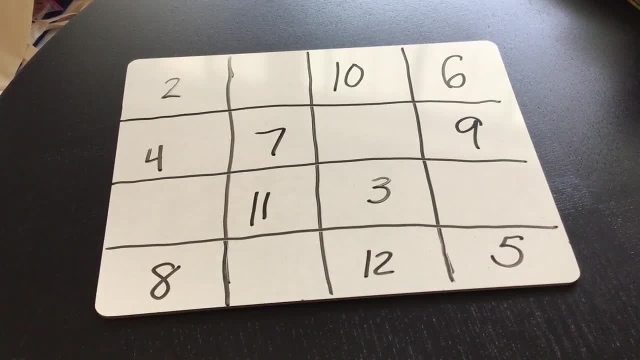 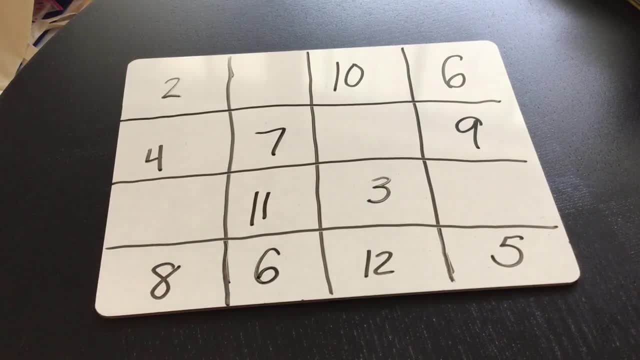 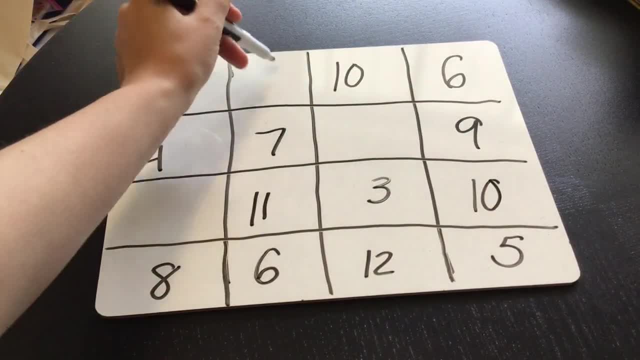 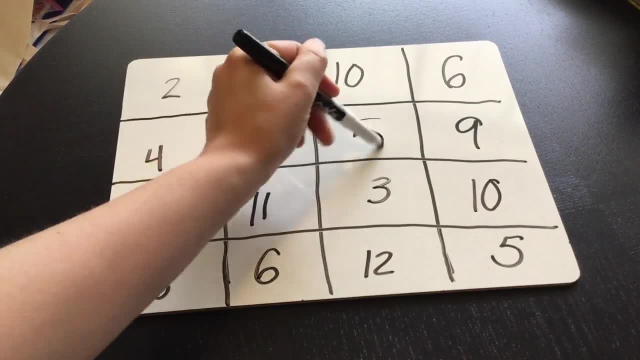 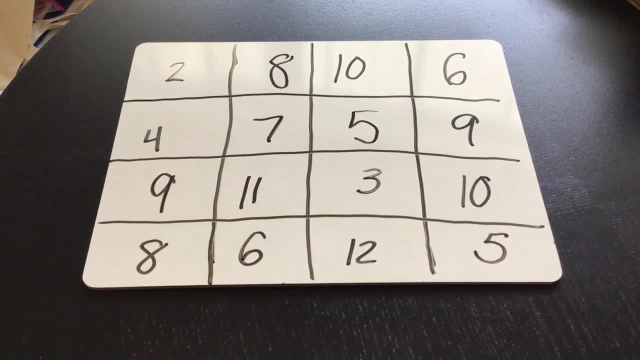 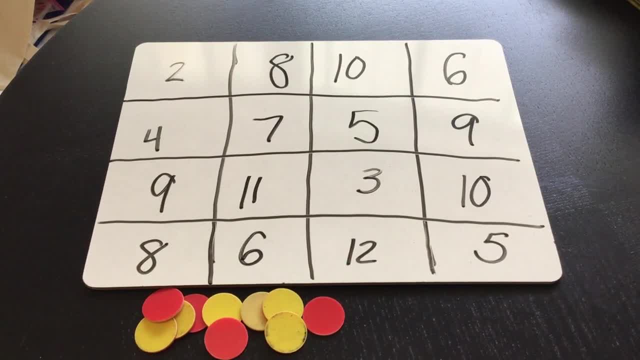 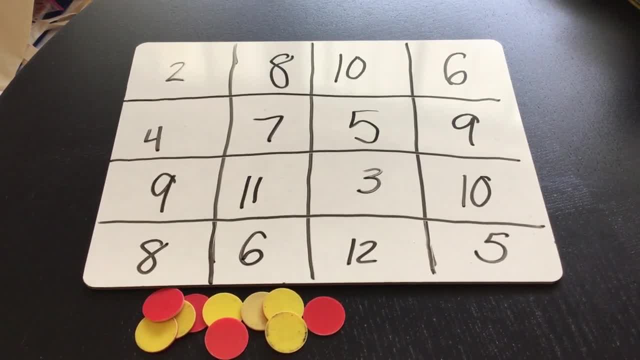 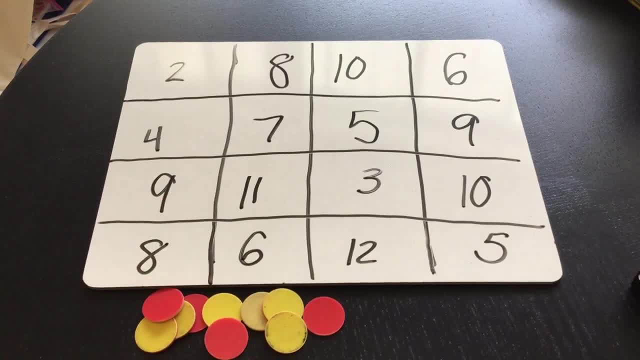 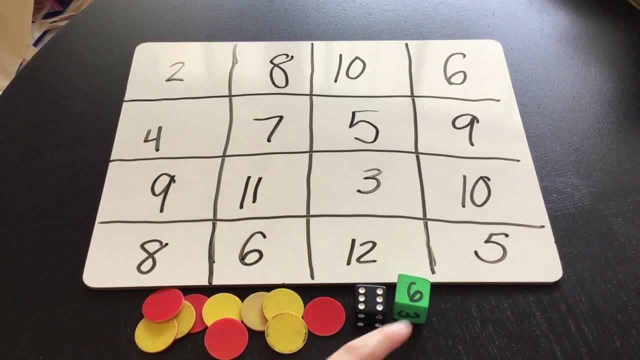 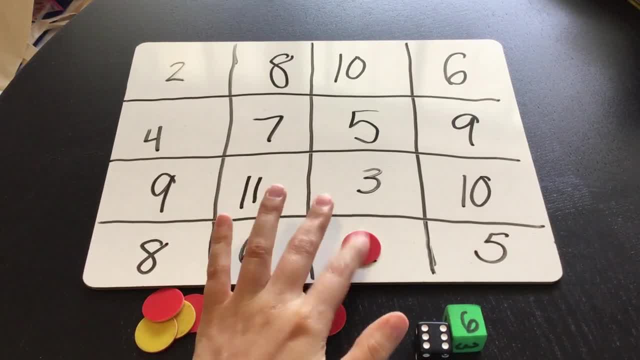 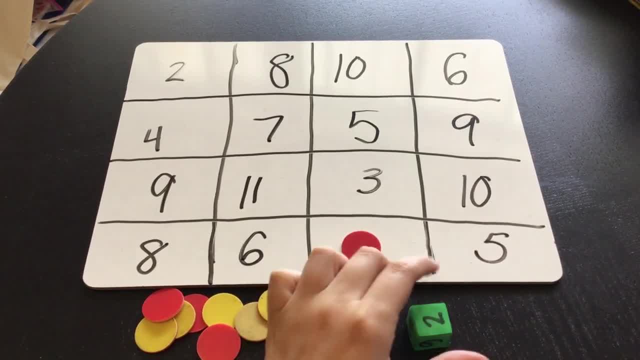 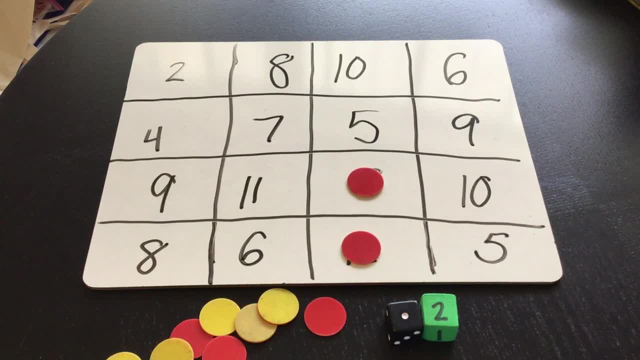 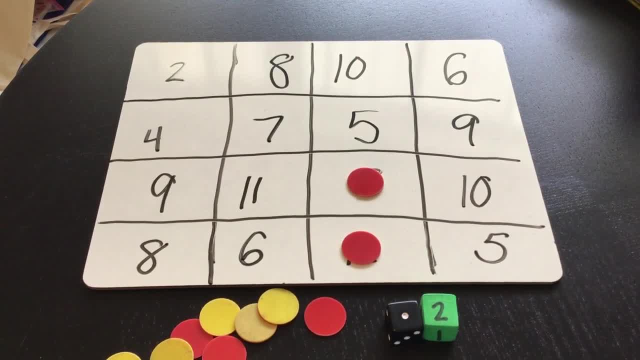 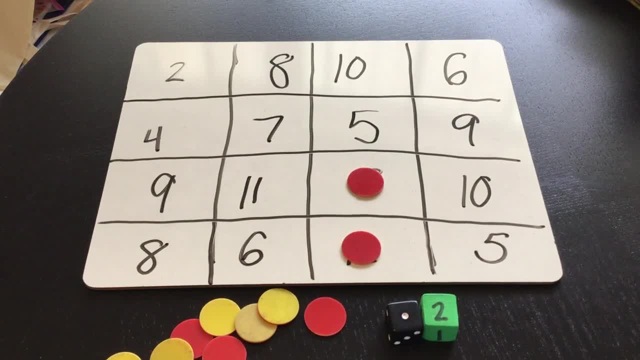 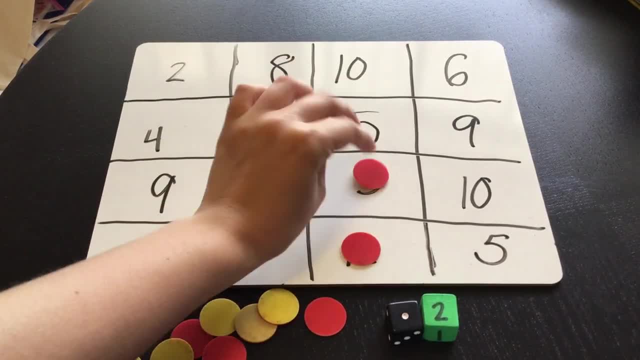 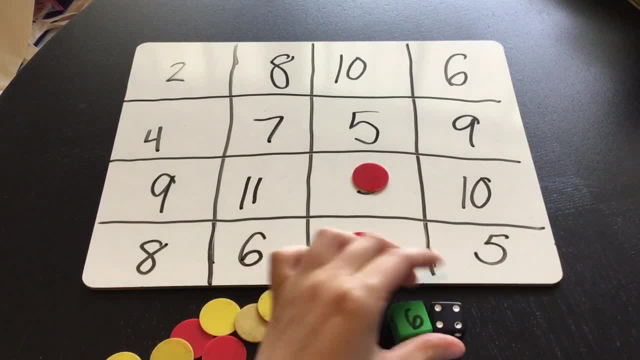 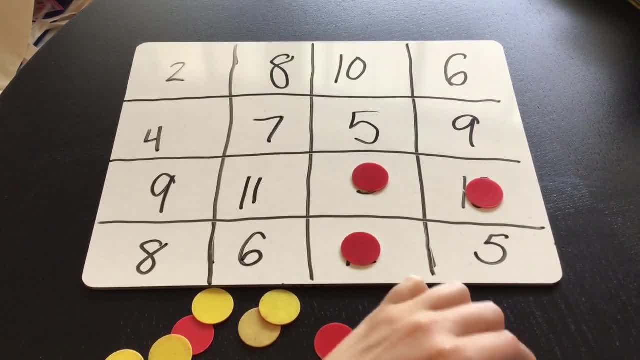 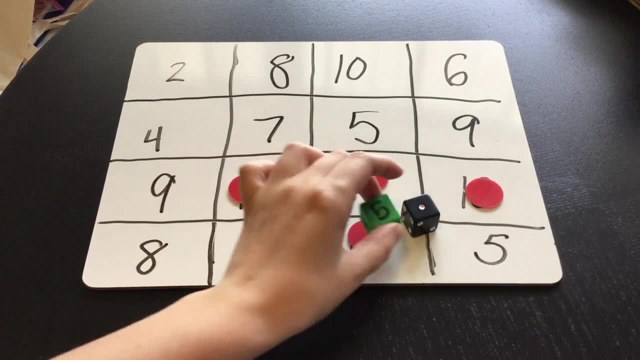 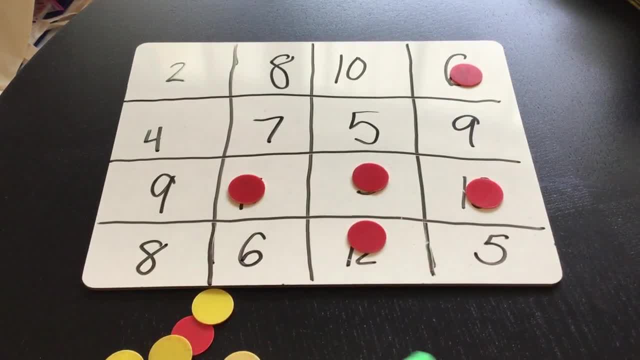 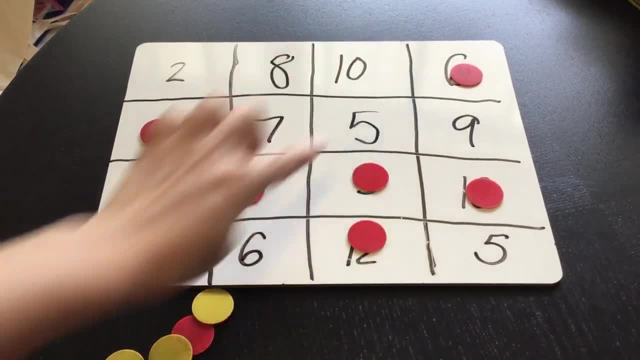 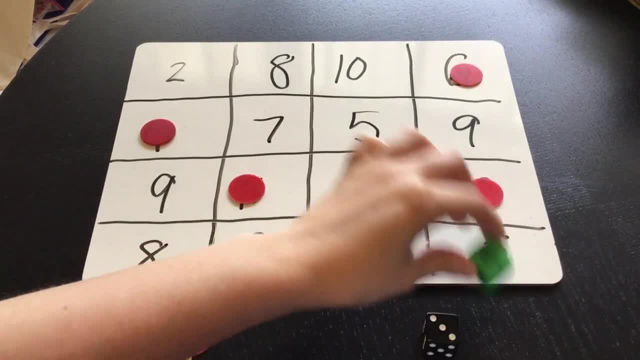 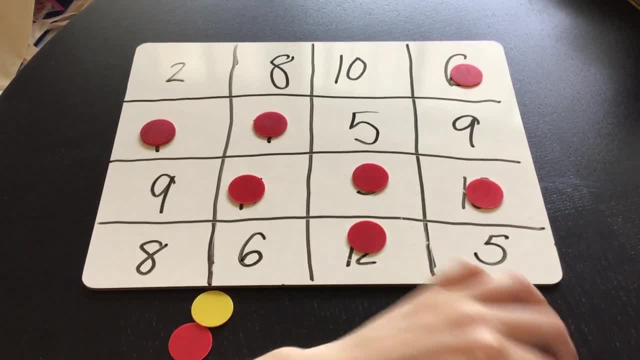 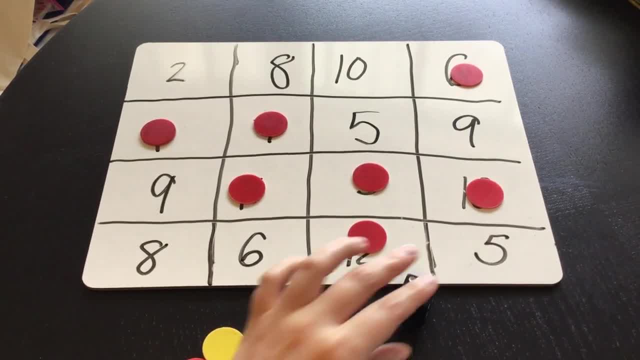 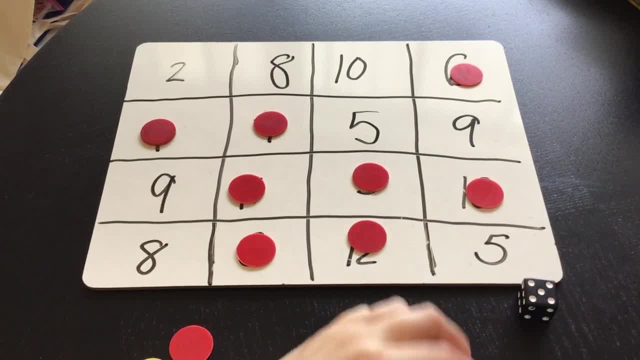 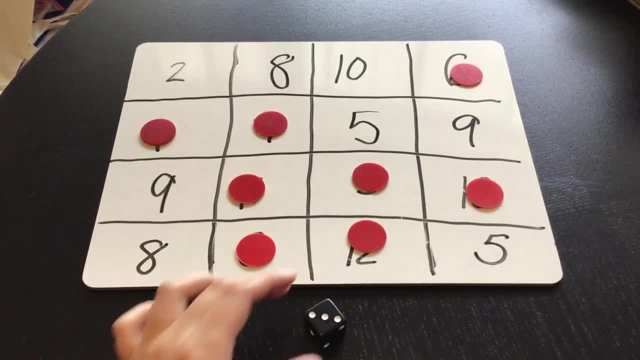 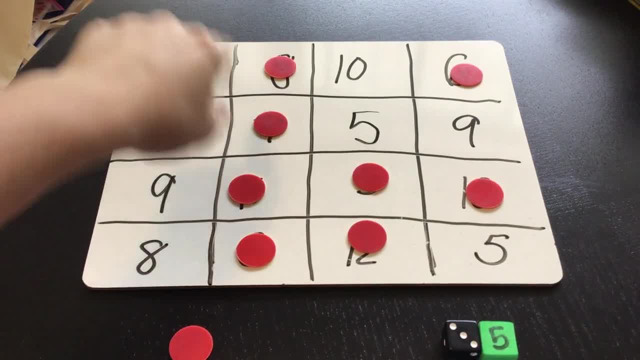 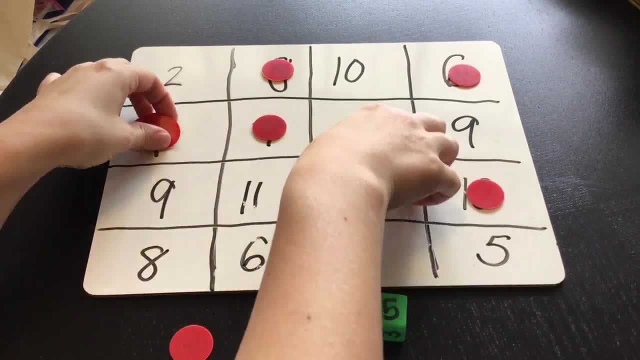 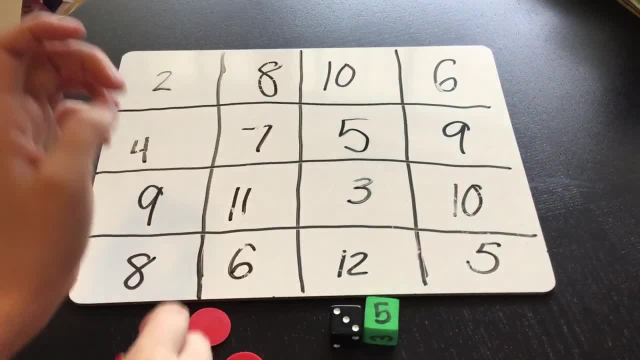 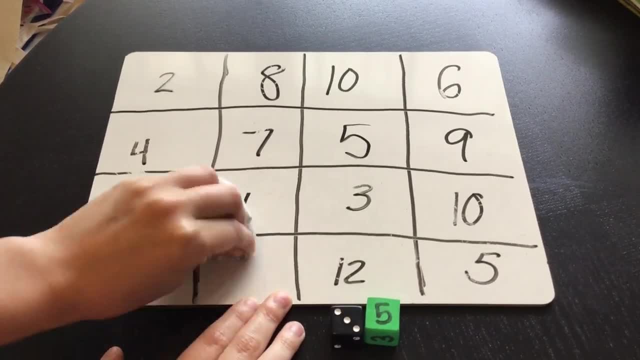 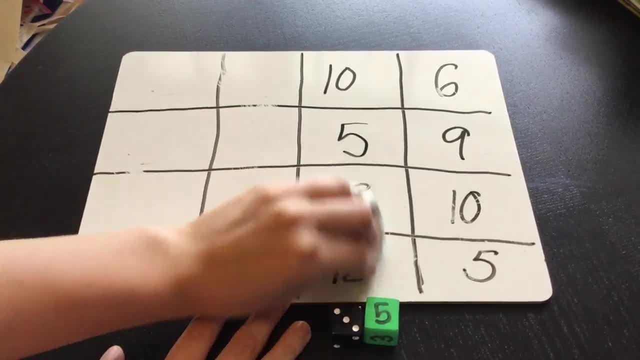 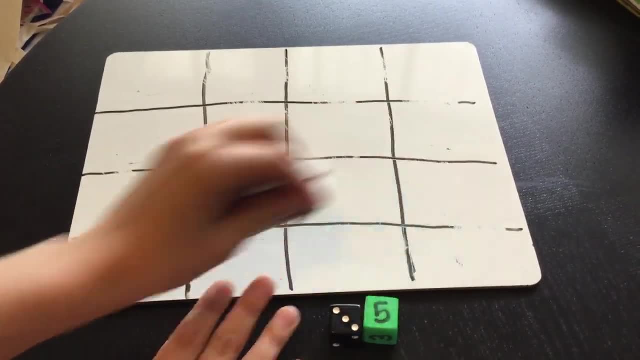 So those are just two. So those are just two. Theそれs I get on the two dice when I roll, When I subtract, are a five, And the lowest number I can get is a zero. And the lowest number I can get is a zero. 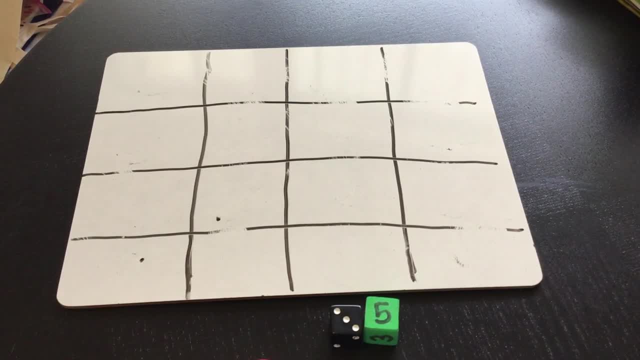 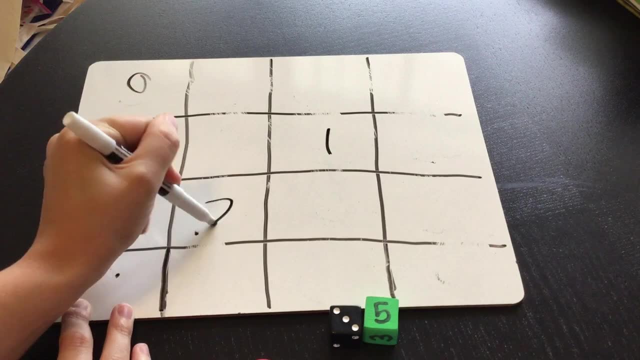 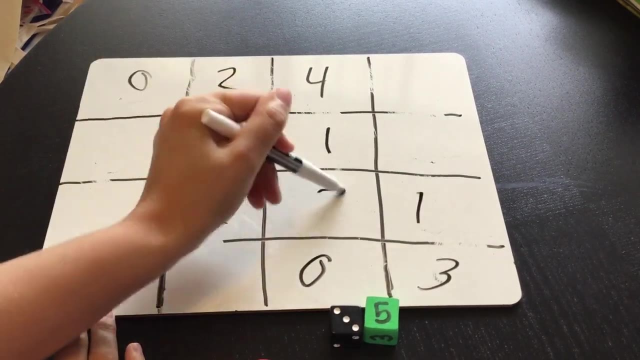 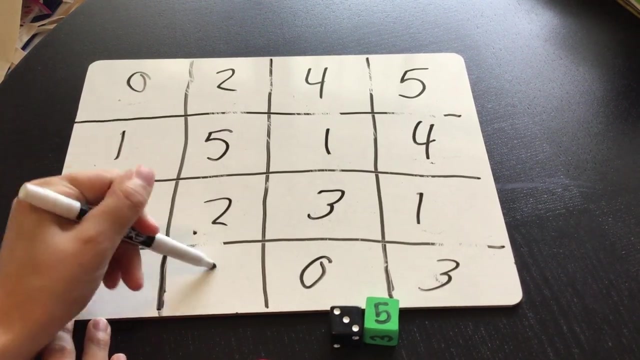 So the good thing about using a whiteboard marker- So the good thing about using a whiteboard marker Is that I can erase and do te except again- Is that I can erase and do te except again. But you can always clear your pieces off. two, three, four, five zero one, two, three, four, five zero one, two, three, okay, so now. 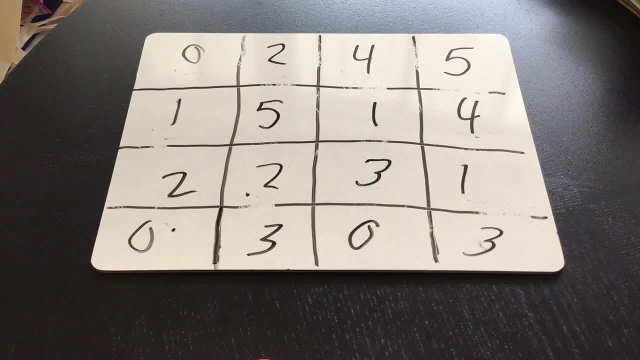 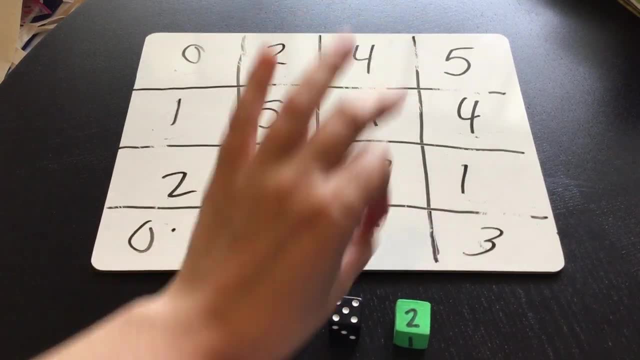 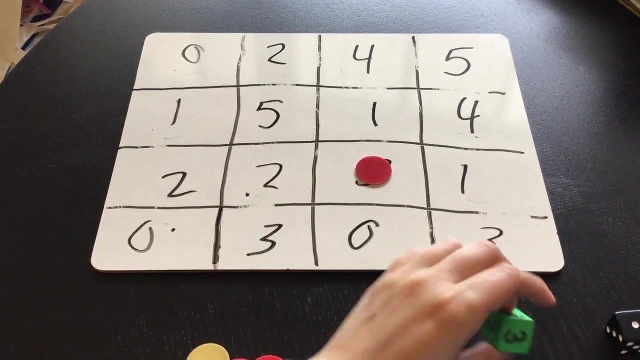 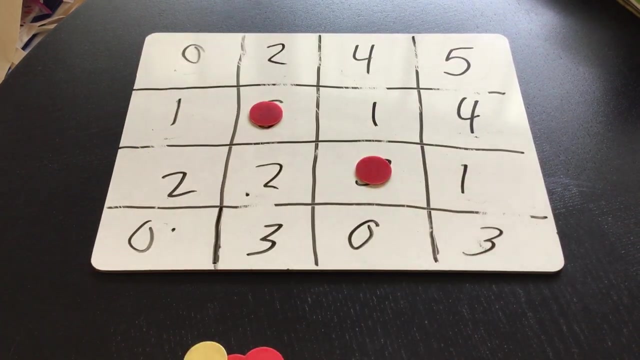 if I'm doing this subtraction game, I roll my two dice. I got five and a two, so five take away. two. five, four, three. I get to cover a three. okay, then I roll again six. oh oh, oh, it was a six. six take away. one is six. five, right, okay, two take away. 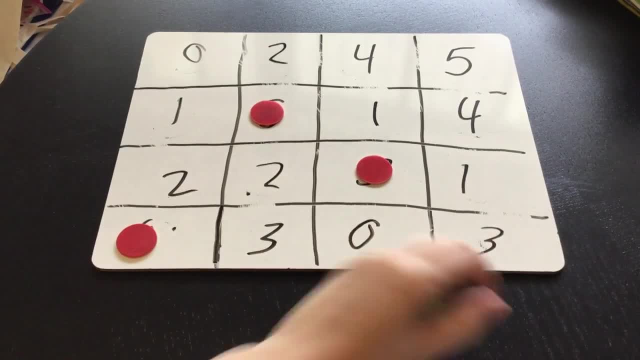 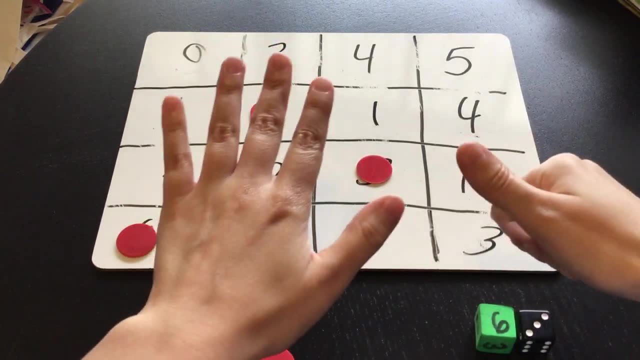 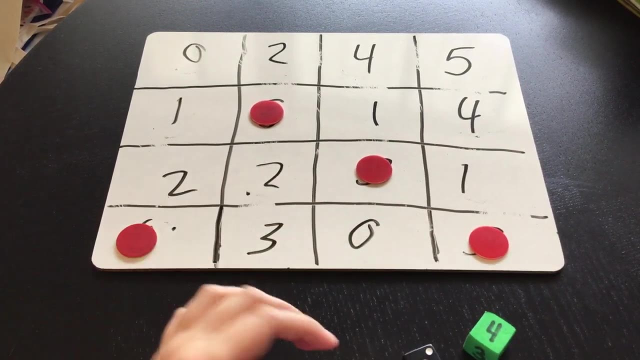 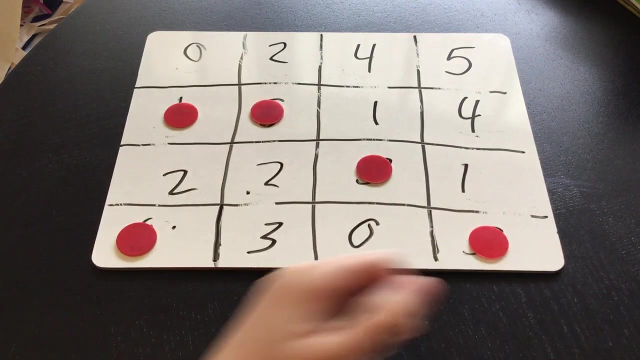 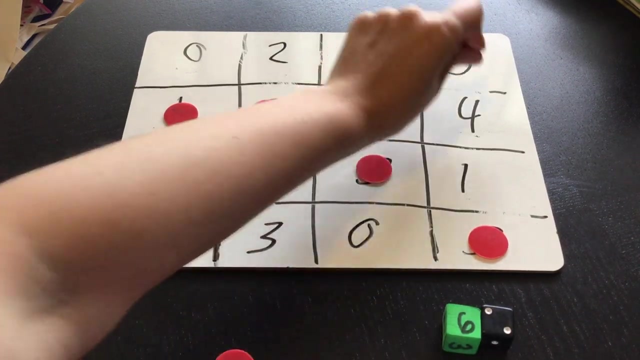 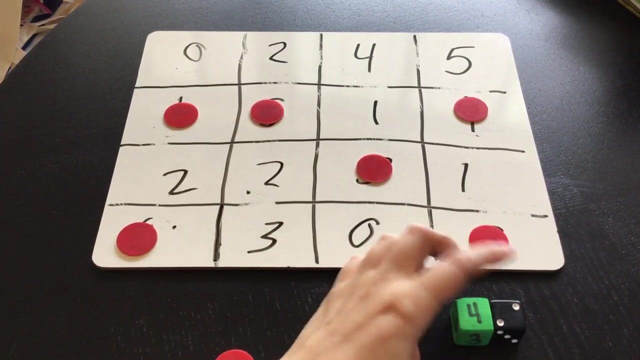 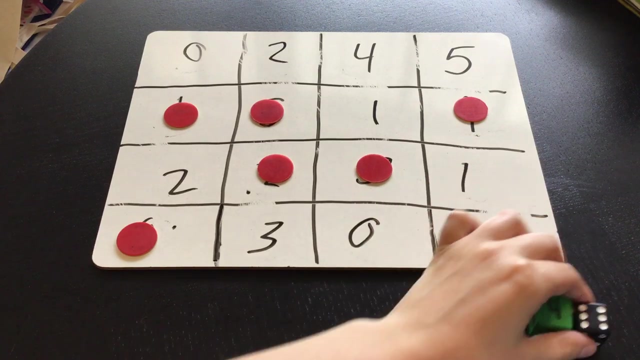 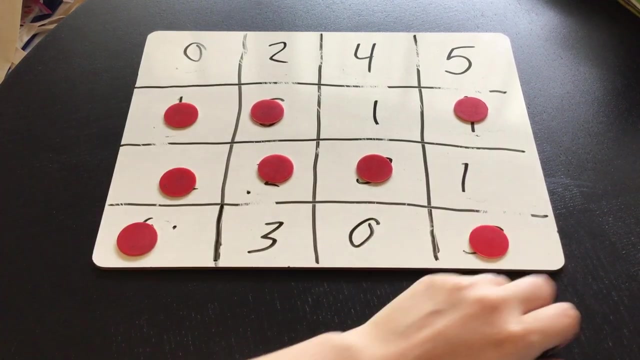 two is zero, six. take away three, six, five, four. three is three, four. take away three, four, three, two, one, six. take away two, six, five, four, four. take away two, four, three, two, six, take away four, six, five, four, three, two. oh, I'm getting close to a couple. 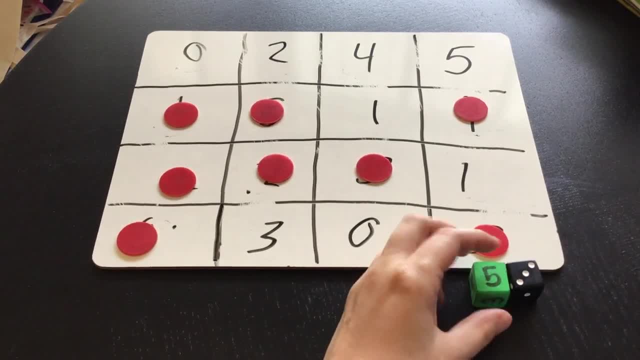 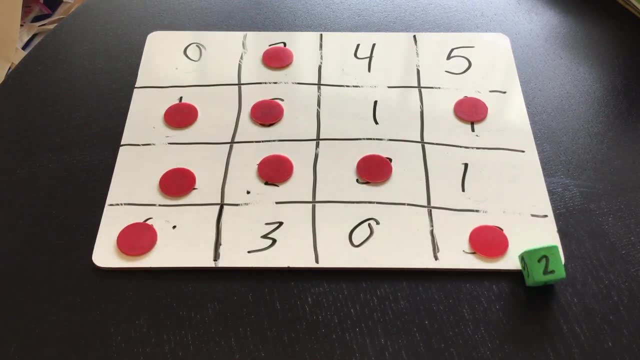 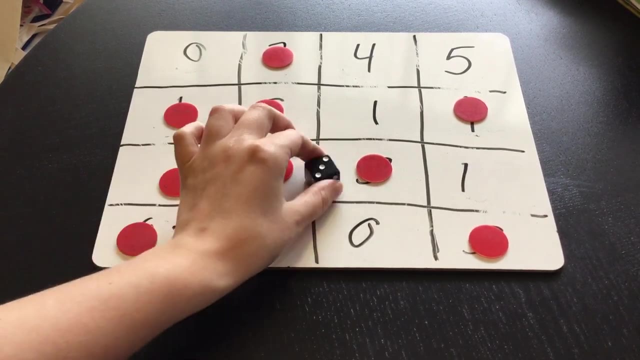 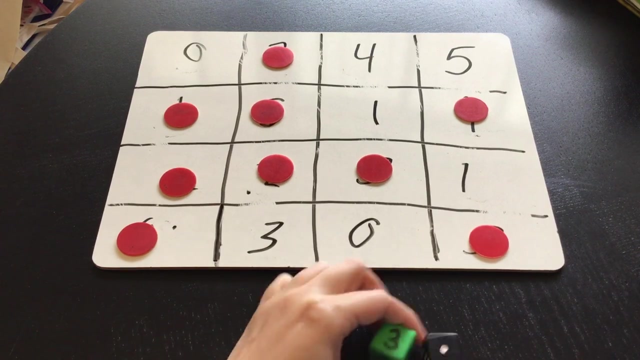 bingos here. right, five take away three, five, four, three, two. I've run out of twos. four take away two, four, three, two, just that I didn't have any two's left. oh, five takeaway three is also two. three take away one is two. oh my goodness, I should have filled my whole.